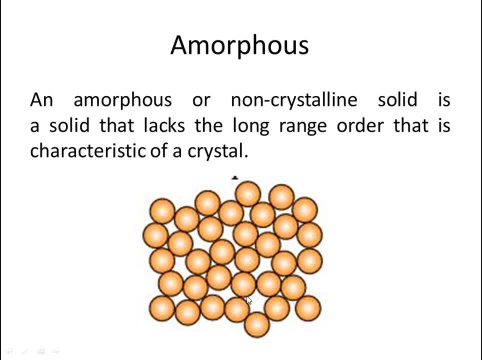 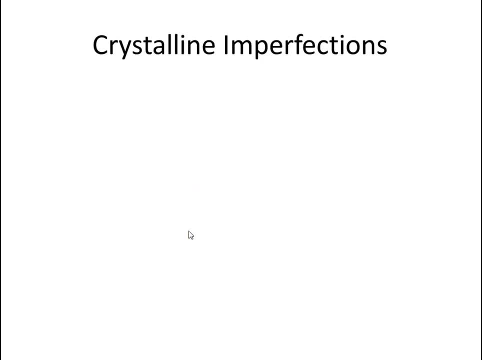 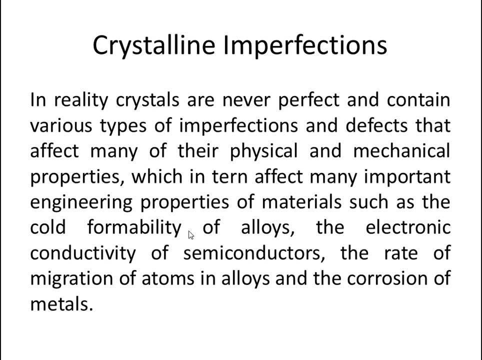 And if we check the figure, that these atoms are not orderly arranged or there is a lack of crystalline structure. And now let's talk about the crystalline imperfections. In reality, crystals are never perfect and contain various types of imperfections and defects that affect many of their physical and mechanical properties. 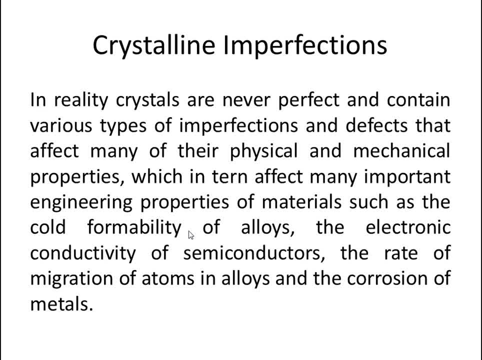 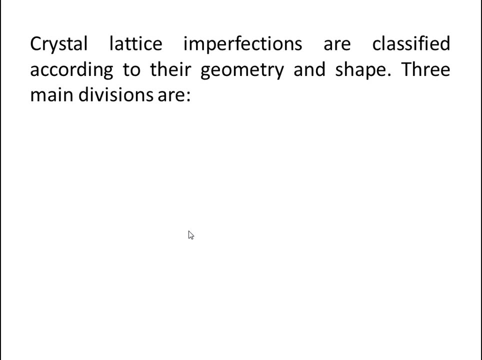 which in turn, affect many important engineering properties of materials, such as the cold formability of alloys, the electronic conductivity of semiconductors, the rate of migration of atoms in alloys and the corrosion of metals. Crystal lattice imperfections are classified according to their geometry and shape. 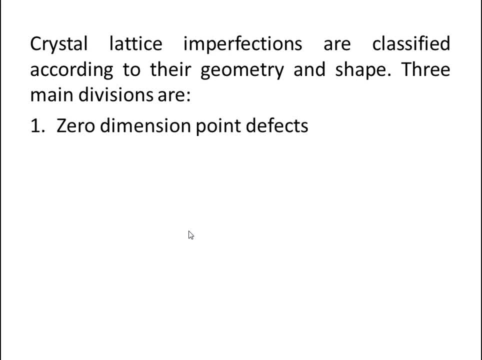 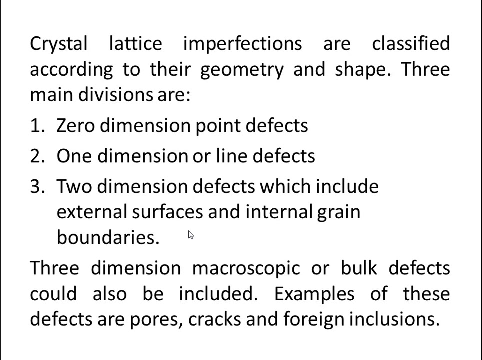 Three main divisions are: First, one zero-dimension point defect. Second one one-dimension or line defects. And third one two-dimension defects, which include external surfaces and internal grain boundaries. Three-dimension, macroscopic or bulk defects could also be included. 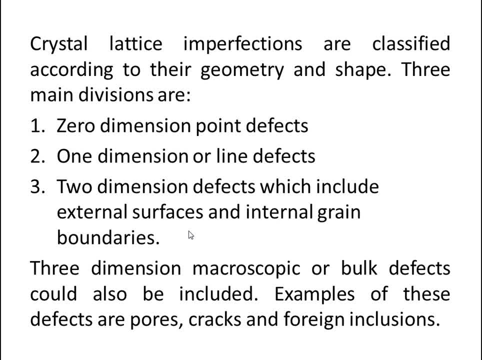 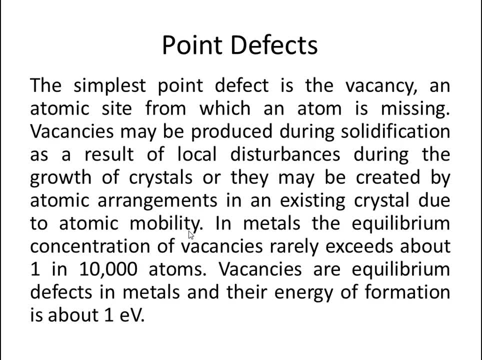 Examples of these defects are pores, cracks and foreign inclusions. Let's talk about point defects. The simplest point defect is the vacancy, an atomic site from which an atom is missing. Vacancies may be produced during solidification, as a result of local disturbances during the growth of crystals. 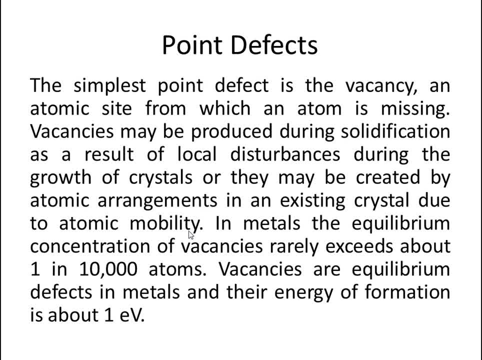 or they may be created by atomic arrangements in an existing crystal. due to atomic mobility In metals, the equilibrium concentration of vacancies rarely exceeds about 1 in 10,000 atoms. Vacancies are equilibrium defects. Equilibrium defects in metals and their energy of formation is about one electron volt. 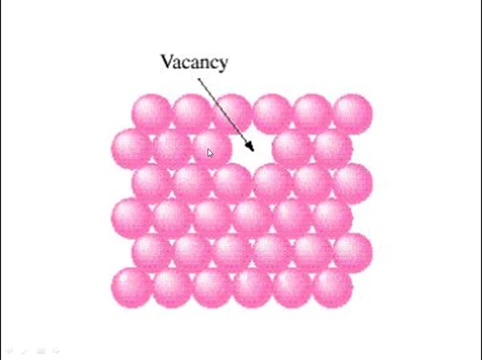 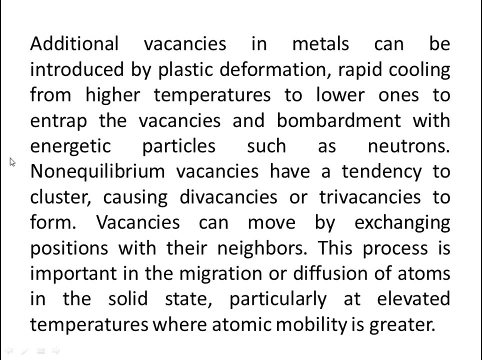 And check this figure, And there is a vacancy And there is a lack of atom. So this is one kind of defect. Additional vacancies in metals can be introduced by plastic deformation, Rapid cooling from higher temperature to lower ones to entrap the vacancies and bombardment with energetic particles such as neutrons. 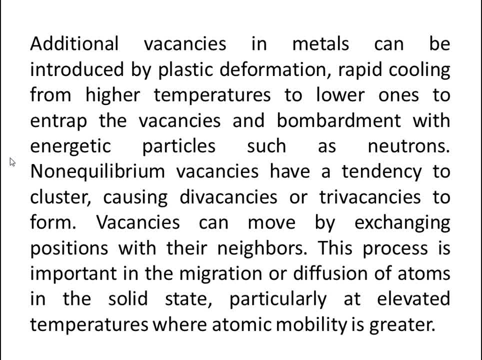 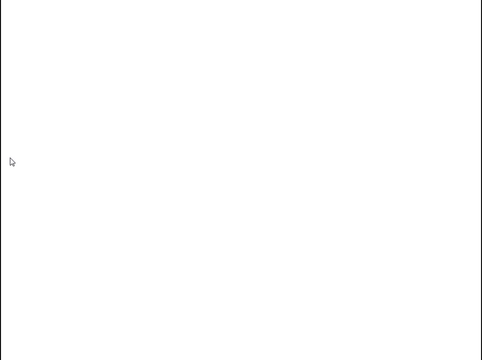 Non-equilibrium vacancies have a tendency to cluster, causing divacancies or trivacancies to form. Vacancies can move by exchanging positions with their neighbors. This process is important in the migration or diffusion of atoms In the solid state. particularly at elevated temperatures, our atomic mobility is greater. 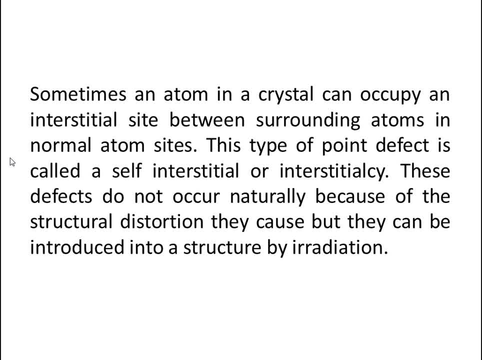 Sometimes an atom in a crystal can occupy an interstitial site between surrounding atoms. in normal atom sites This type of point defect is called a self-interstitial or interstitiality. These defects do not occur naturally because of the structural distortion they cause, But they can be introduced into a structure by irradiation. 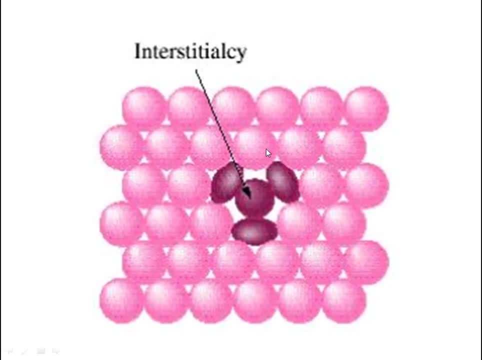 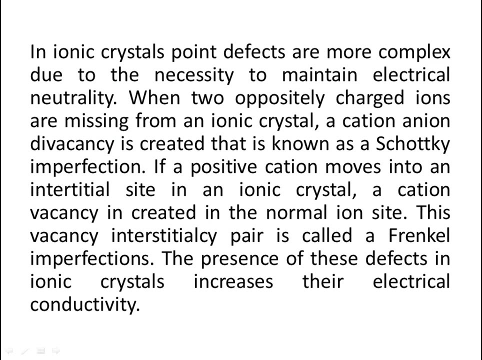 And this is the defect, And this is called interstitiality. In ionic crystals. point defects are more complex due to the necessity to maintain electrical neutrality. When two oppositely charged ions are missing from an ionic crystal, a cation-anion divacancy is created. that is known as a Schottky imperfection. 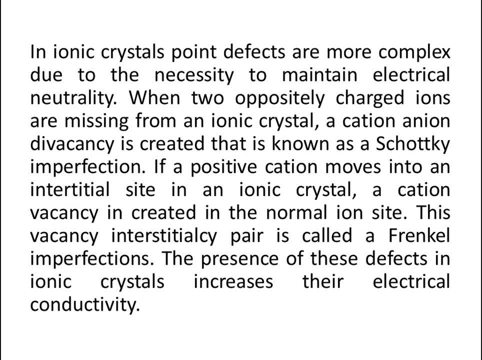 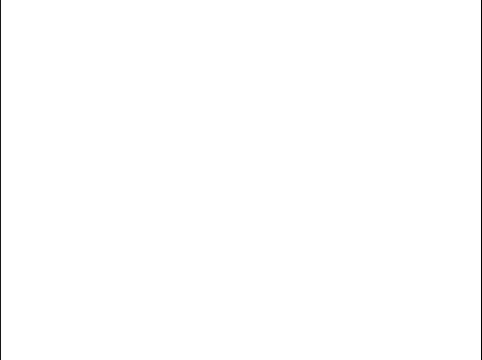 In a positive cation moves into an interstitial site in an ionic crystal, a cation vacancy is created in the normal ion site. This, I can say interstitial CPR, is called a Frankel imperfection. The presence of these defects in ionic crystals increases their electrical conductivity. 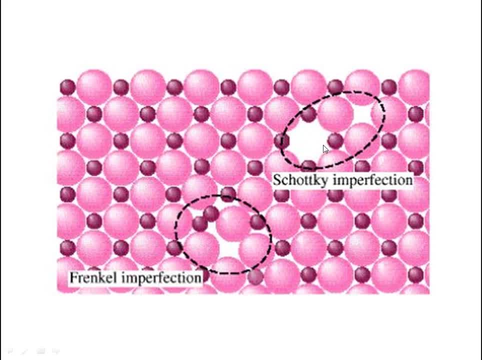 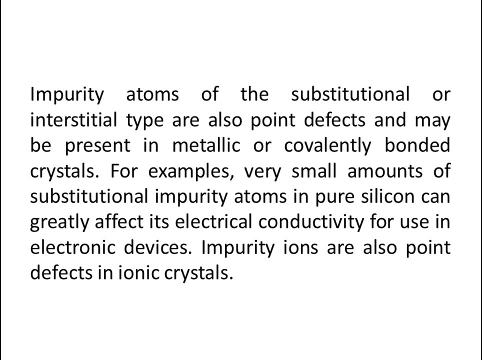 And check this figure. So this imperfection is called Schottky imperfection And this imperfection is called Frankel imperfection. Impurity atoms of the substitutional or interstitial type are also point defects and may be present in metallic or covalently bonded crystals. 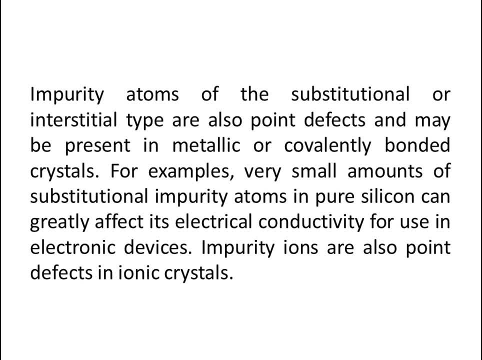 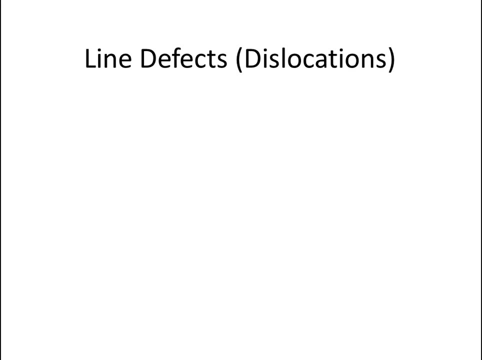 For examples, very small amounts of substitutional impurity atoms in pure silicon can greatly affect its electrical conductivity for use in electronic devices. Impurity ions are also point defects In ionic crystals, And let's talk about line defects, That is, dislocations. 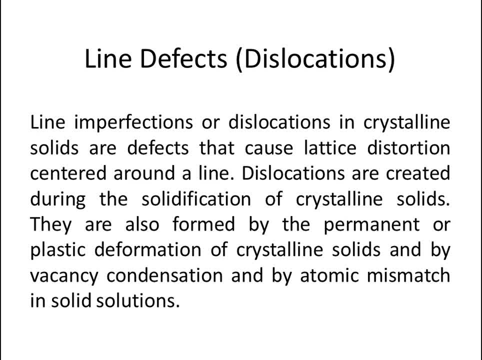 Line imperfections or dislocations in crystalline solids are defects that cause lattice distortion centered around a line. Dislocations are created during the solidification of crystalline solids. They are also formed by the permanent or plastic deformation of crystalline solids and by vacancy condensation and by atomic mismatch in solid solutions. 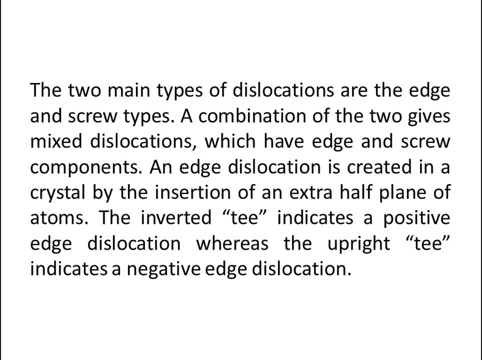 The two main types of dislocations are the edge and screw types. A combination of the two gives mixed dislocations which have edge and screw components. An edge dislocation is created in a crystal by the insertion of an extra half plane of atoms. 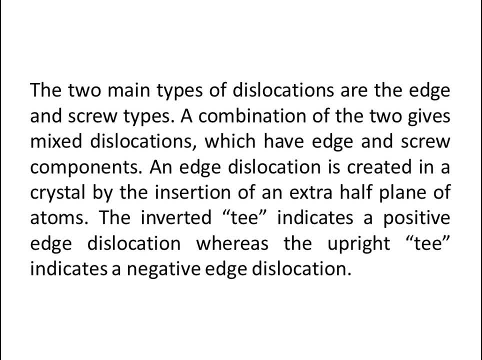 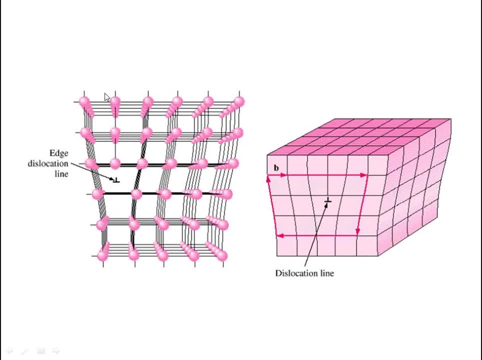 The inverted T indicates a positive edge dislocation, whereas the upright T indicates a negative edge dislocation, And check this figure. So this is edge dislocation. So this line has been finished here. And this is another edge dislocation, So this line has been finished. 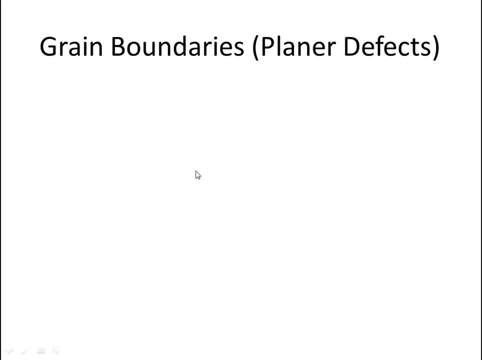 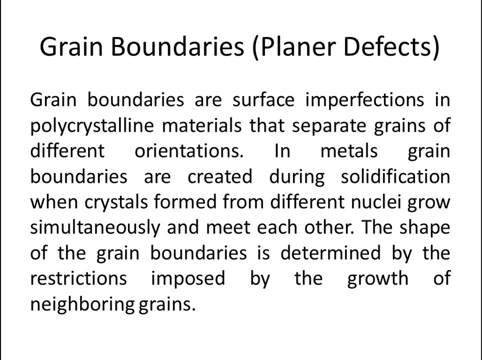 So this line has been finished here And let's talk about grain boundaries. that is called planar defects. Grain boundaries are surface imperfections in polycrystalline materials that separate grains of different orientations. In metals, grain boundaries are created during solidification.